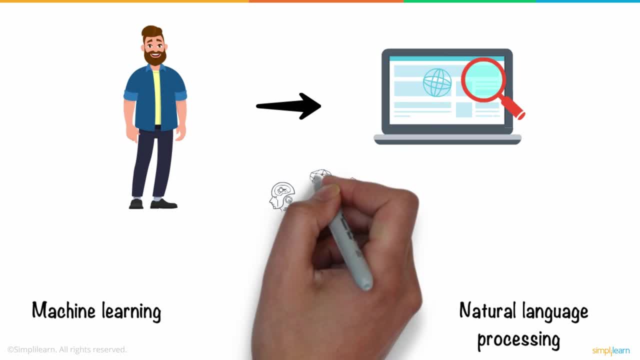 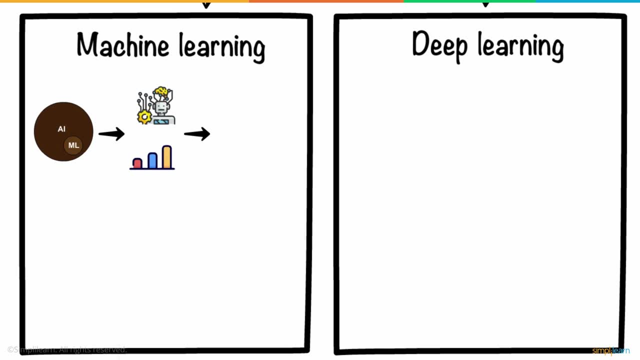 deep learning and natural language processing are all connected with artificial intelligence. Machine learning, a subset of AI, is the process of automating and enhancing how computers learn from their experiences without human help. Machine learning can be used in email, spam detection, medical diagnosis, etc. Deep learning can be considered a subset of machine learning. 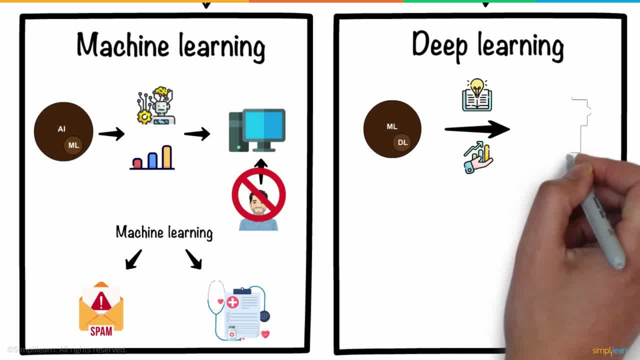 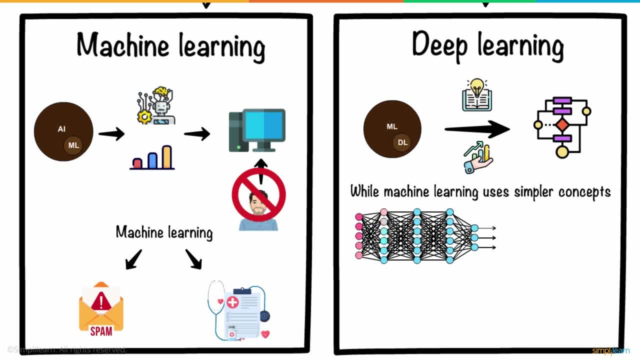 It is a field that is based on learning and improving on its own by examining computer algorithms. While machine learning uses simpler concepts, deep learning works with artificial neural networks which are designed to imitate artificial intelligence. Machine learning is not just a tool to imitate the human brain. This technology can be applied in face recognition. 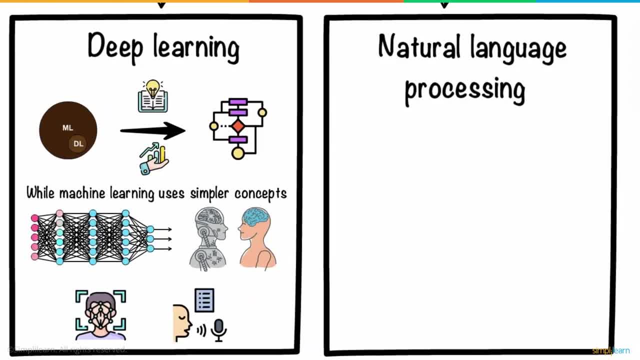 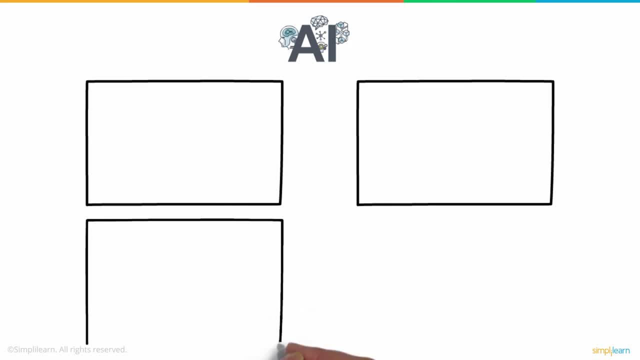 speech recognition and many more applications. Natural language processing, popularly known as NLP, can be defined as the ability of machines to learn human language and translate it. Chatbots fall under this category. Artificial intelligence is advancing in every crucial field, like healthcare, education, robotics, banking, e-commerce, and the list goes on. Like in healthcare. 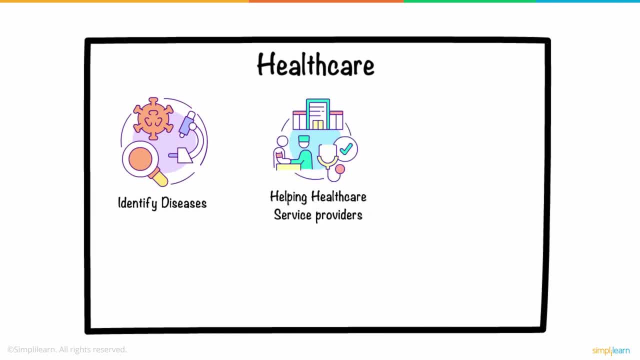 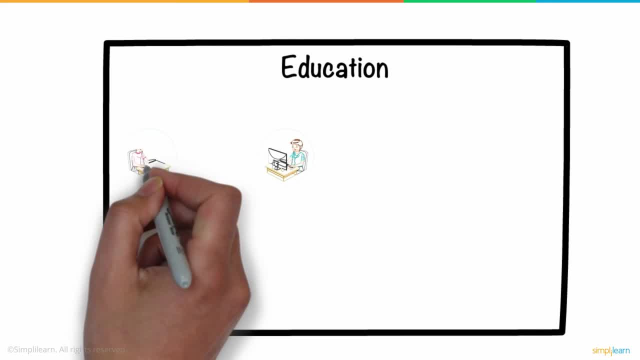 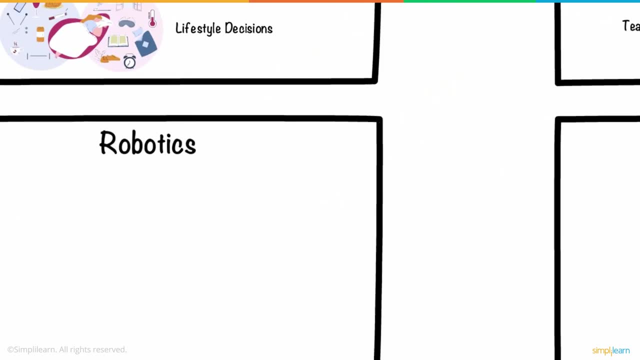 AI is used to identify diseases, helping healthcare service providers and their patients make better treatment and lifestyle decisions. Coming to the education sector, AI is helping teachers automate grading, organizing and facilitating parent-guardian conversations In robotics. AI-powered robots employ real-time updates to detect obstructions in their path. 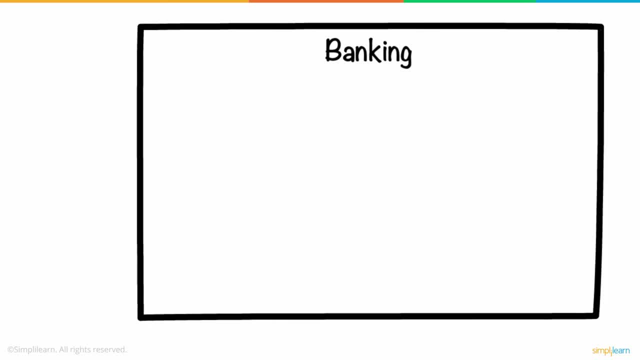 and instantaneously design their routes. Artificial intelligence provides advanced data analytics. that is transforming banking technology and education. AI is used to identify diseases, helping healthcare service providers and their patients make better treatment and lifestyle decisions. Coming to the education sector, AI is helping teachers automate grading. 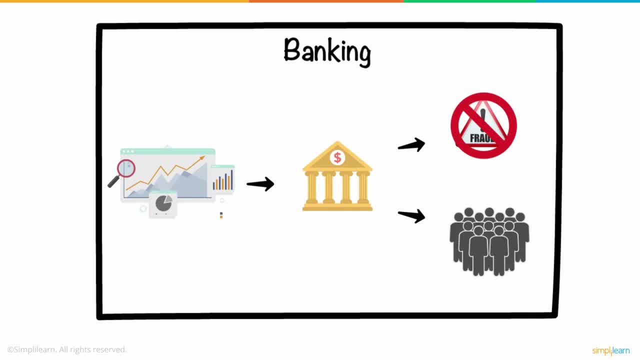 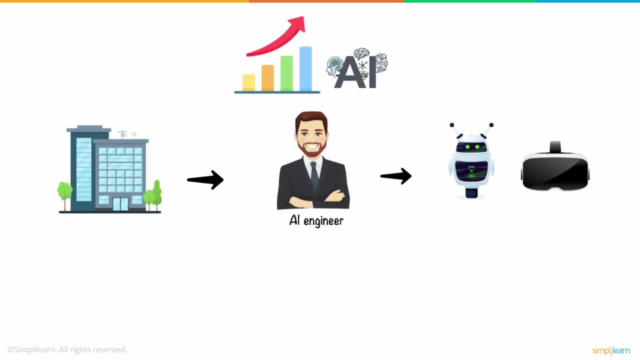 design and facilitate parent-guardian conversations. With this growing demand for AI, more and more industries are looking for AI engineers who can help them develop intelligent systems and offer them lucrative salaries going north of $120,000.. The future of AI looks promising, with the AI market expected to reach $190 billion by 2025.. 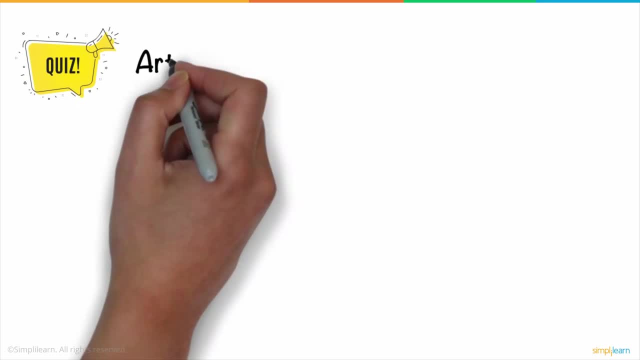 So, on that note, I have a question for you. Artificial intelligence is about playing a computer game, or playing a game of chess, or playing a game of chess, or playing a game of chess, or playing a computer game: Creating a device using your own intelligence.